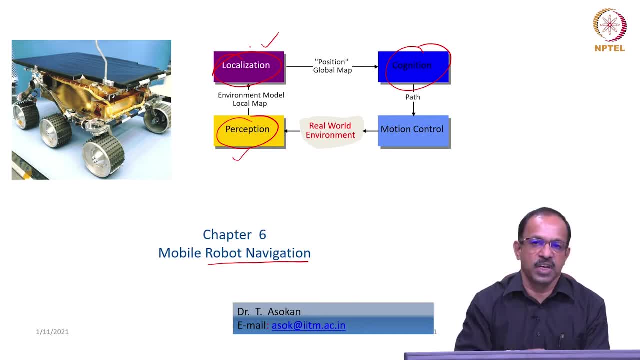 So, once the robot is clear about its location and it has already been given an instruction to go to a particular target, the next task is basically within the known position, with the known position of the robot in the map, how the robot will actually plan. 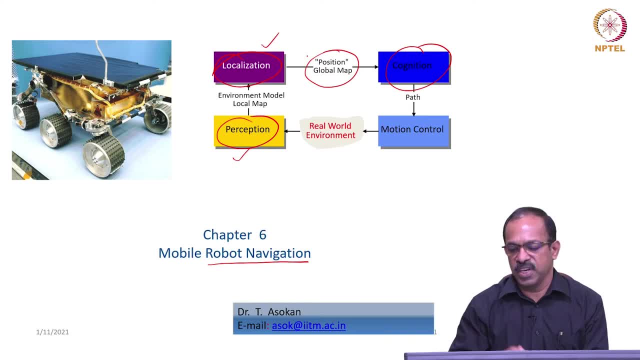 its path to reach its target. So this stage is basically known as the cognition stage, where the robot will utilize all the information it has, including the information given by the user, as well as the information collected by the sensors or through the sensors. the robot will start using this information and then 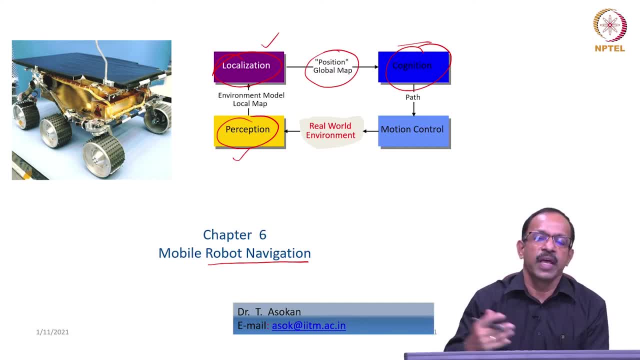 decide on what is the next course of action or how it should actually execute or plan for its next course of action. So that is basically using the information and then making decision is basically the cognition stage. So the cognition stage will help the robot to 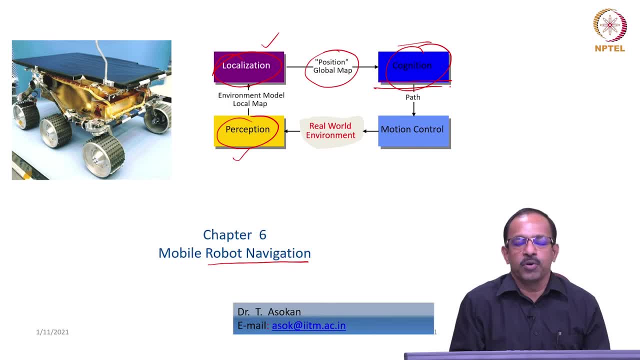 decide a path which it need to follow in order to reach its target. So that is basically the path will be generated. So this stage of generating a path and then following the path to reach its target is basically known as the mobile robot navigation. So the robot need to 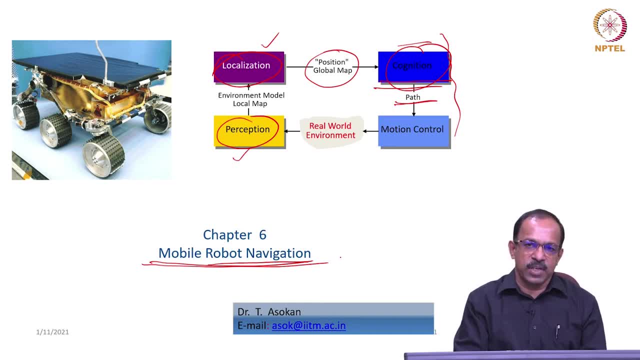 navigate from its current location to the target location using the information it collected and the information it has based about its location, and then use all this information and then plan a path and then reach the goal. So once you plan path is planned, then basically the motion control will help the robot to follow that path and then reach its 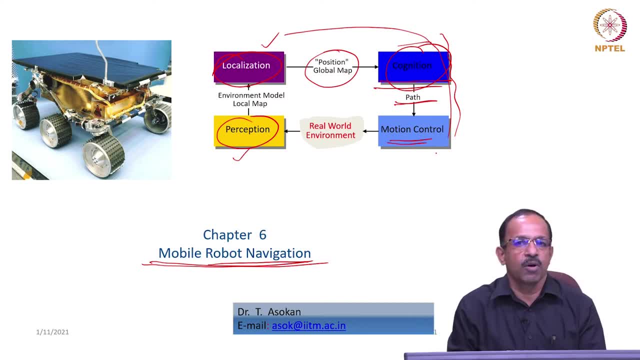 target. So this is the steps involved in autonomous motion of a robot. So today we will look into the mobile robot navigation and what are the various steps involved in navigating a robot from a known location to a target location. So the first part: we look at the navigation today in the first lecture. 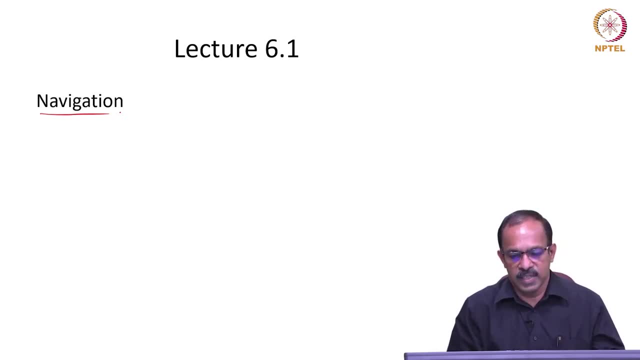 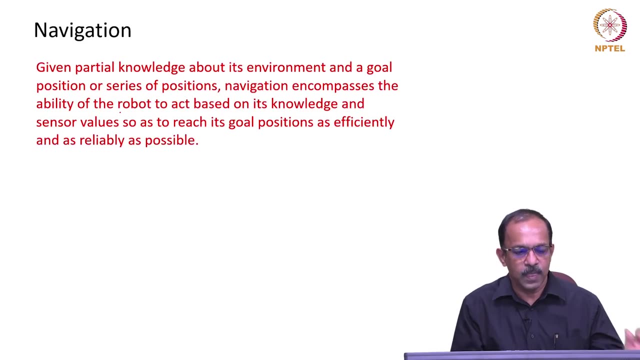 we will look at the navigation and various steps involved in navigation And as we progress we look into more aspects of navigation of the robots. So now the navigation is defined as given a partial knowledge about its environment and a goal position or a series of positions. The navigation encompasses the ability of the 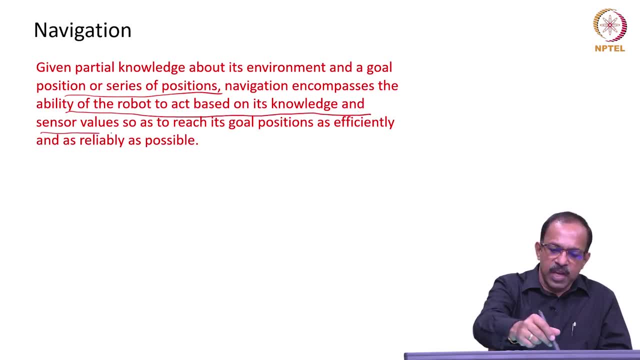 robot to act based on its knowledge and sensor values, so as to reach its goal position as efficiently and as reliably as possible. So that is basically the navigation of a robot, So it knows the information about its current position and it has got sensors. 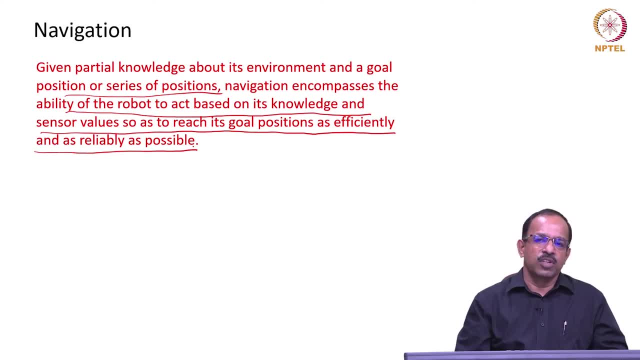 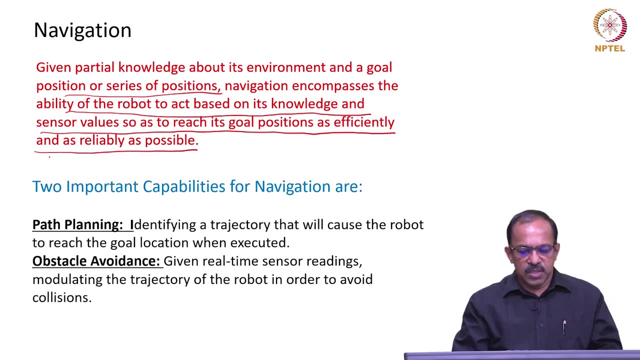 to collect information and, with all these, how the robot will actually move from its current location to and reach its goal position as efficiently and as reliably as possible is basically known as the navigation, And this involves two important capabilities for robots. The first one is we call this as the path planning. 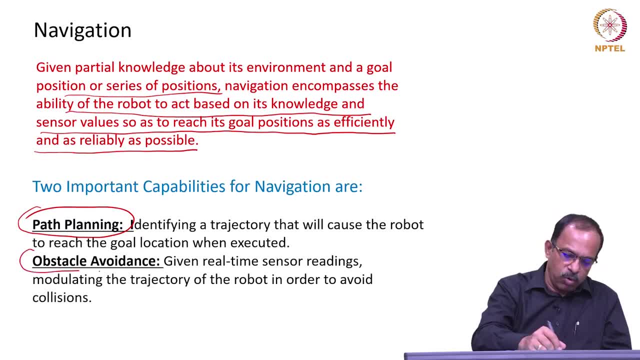 And the second one is obstacle avoidance. So if the robot has to navigate, first it needs to plan a path from current location to the target location, or to the target locations or via points, and that is basically the planning of the path. So it will be identifying a trajectory that will cause the robot to reach the goal location. 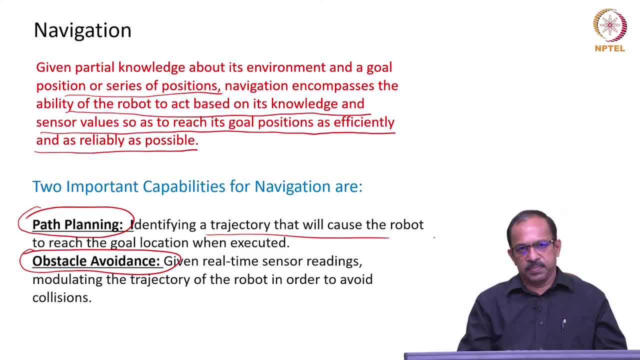 when executed. So that is basically the path planning. The next one is, as the robot moves on its path, it has to avoid obstacles also. so that is basically the obstacle avoidance: Given a real time sensor reading, how to modulate the trajectory of the robot in order to avoid. 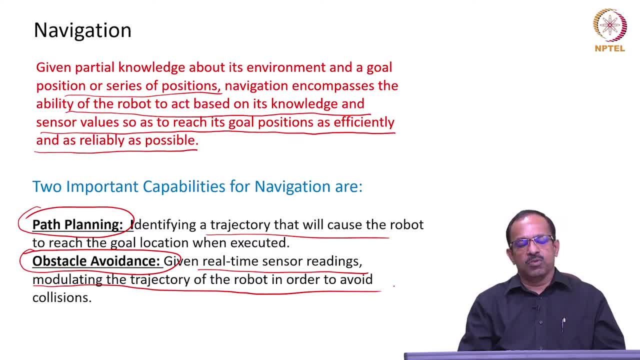 collisions. that is basically the obstacle avoidance. So these are the two capabilities for the robots to be autonomous, that is, it needs to have a capability to plan the paths and then avoid the path, avoid the obstacles as the robot moves along the path. 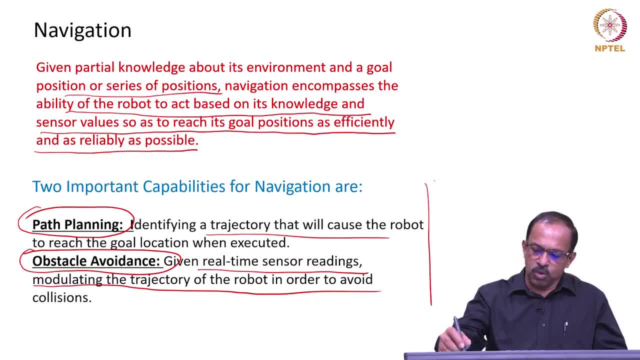 So these are the two capabilities the robot need to have in order to do the navigation. So when we talk about the path planning, then there is a term: trajectory. So path planning and trajectory planning are slightly different. Basically, path planning will talk only about the paths, the points x, y, theta for the 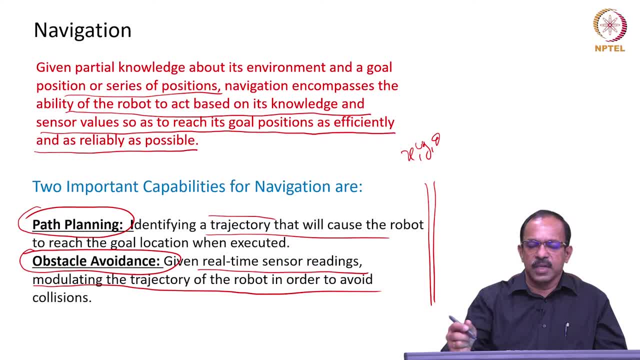 robot. that is basically the path points. The trajectory basically talks about the time at which the robot reach this particular point. So that is basically the trajectory, this particular point. So trajectory is basically a path. information, along with its temporal information, is basically known as the trajectory, Because in the practical scenario, you want the 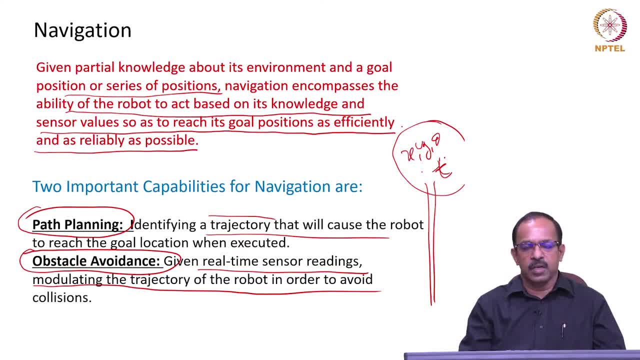 robot to reach a particular location at a particular time or in a particular duration of time. So that is basically the trajectory. Otherwise it is only there is no time. information is not there, then we call it as a path, Otherwise we call it with time information. 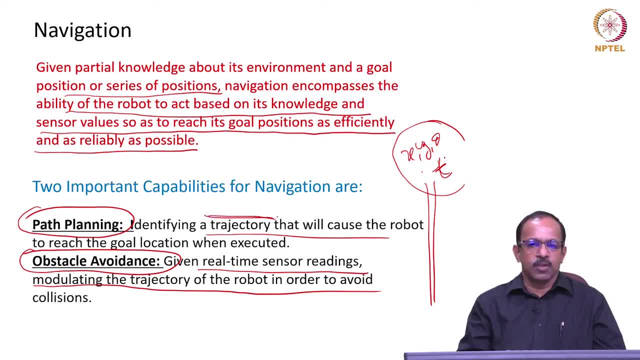 we will call it as the trajectory. So, effectively, the robot finally need to have the trajectory so that it will reach the target at a particular time or the desired time, And as it moves there may be obstacles coming which was not anticipated or which was not there in the 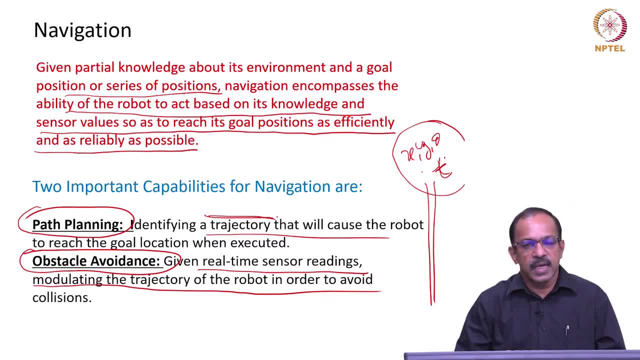 map already available. In that case, the robot needs to replan its trajectory or modulate the trajectory and then avoid the obstacle and reach the target, So that, basically, the obstacle avoidance capability, So these two capabilities need to be built into the robot in order to have an autonomous 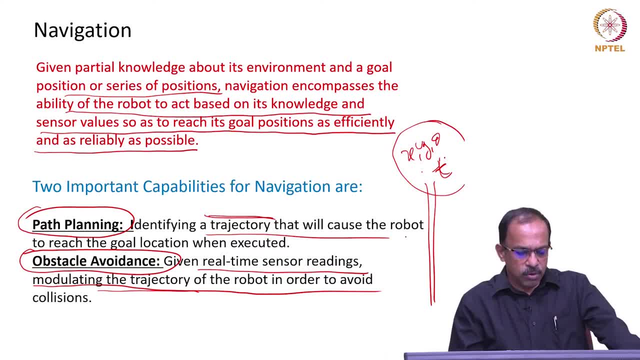 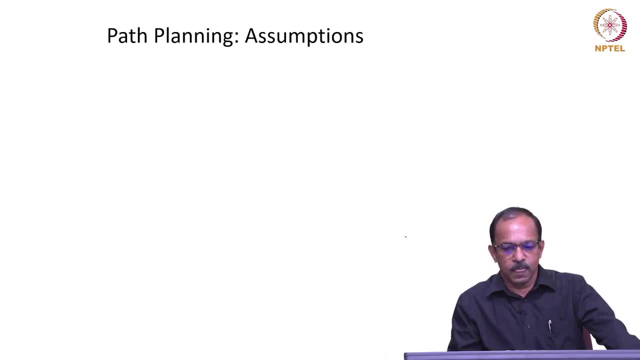 navigation of the robot. So we will look at the path planning initially and then we talk about obstacle avoidance also. So when we do this planning of a path for a robot, we make few assumptions, basically to make our life easier or without too much of complications in the planning. 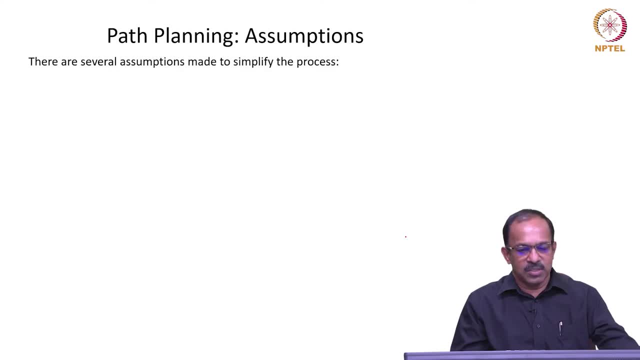 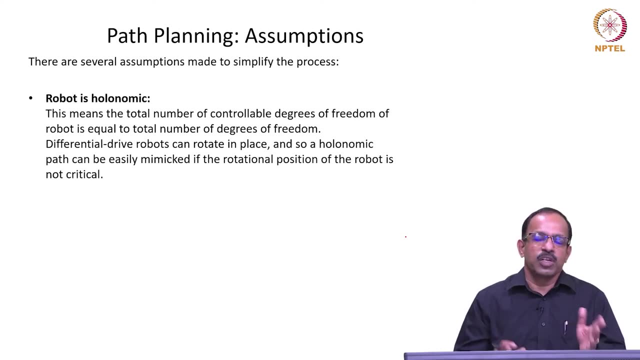 stage We assume that the robot is basically a holonomic one. So holonomic robot is that the robot can actually move the way it wants. So it has got enough degrees of freedom, enough controllable degrees of freedom as the number of degrees of freedom of the robot. So the 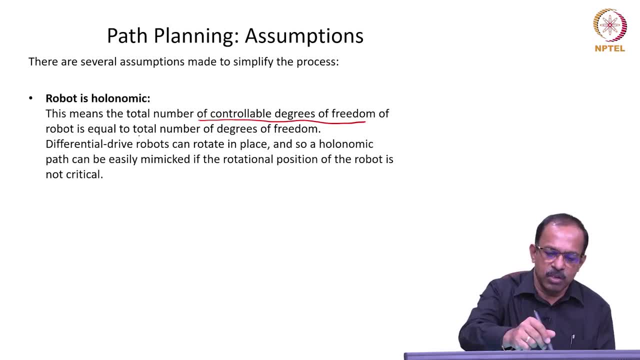 total number of controllable degrees of freedom is equal to the total number of degrees of freedom, So that any object will be having its own degrees of freedom when the ground robot has got its own degrees of freedom, But an aerial robot will be having a different number of degrees of freedom. 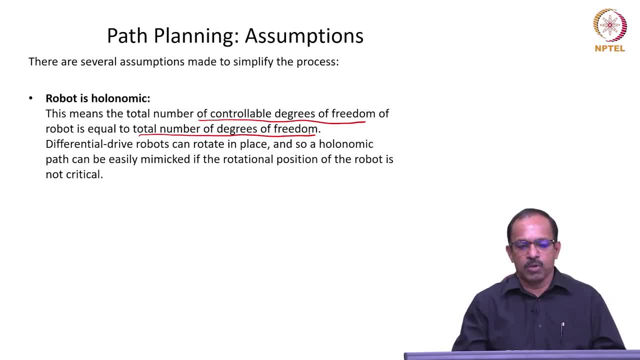 If you can control all those degrees of freedom, then we call it as a holonomic robot. So the robot will be considered as holonomic as long as we can control all the degrees of freedom. That is, nothing is independent. I mean nothing is dependent on the other degrees of freedom, all. 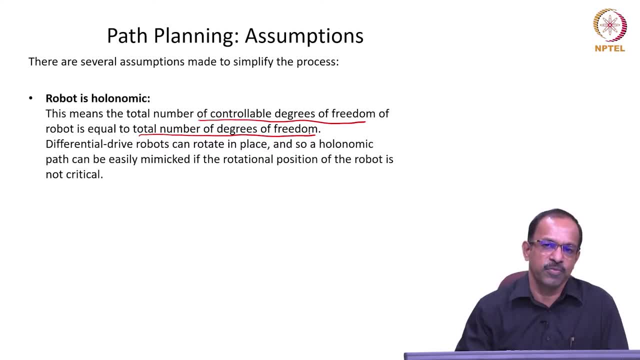 the degrees of freedom are independent and we can control. So that kind of an assumption is basically the assumption is that the whole of the law is independent. So the assumption is that the assumptions are so basic and liberal. So a logical mgantas and the control of one household district in the 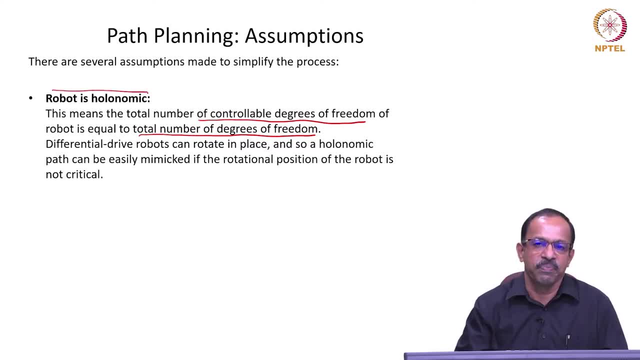 krijamb organic are independent from the other. cos�� pl hacemos. so we can take the same rule to beaches in the that the robot is holonomic. That means the robot can take a turn at its own location. it can move on sideways whenever it needs to move in sideways or a lateral motion is needed. 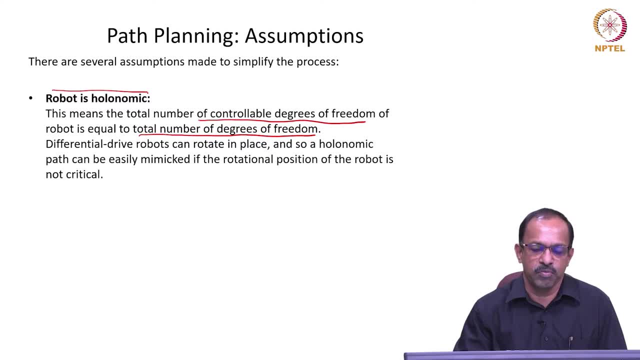 the robot will be able to do that. That is basically the assumption of holonomy. Then another assumption is that it is simply a point. So we assume that the robot is a point. its size is not critical, we assume it is a. 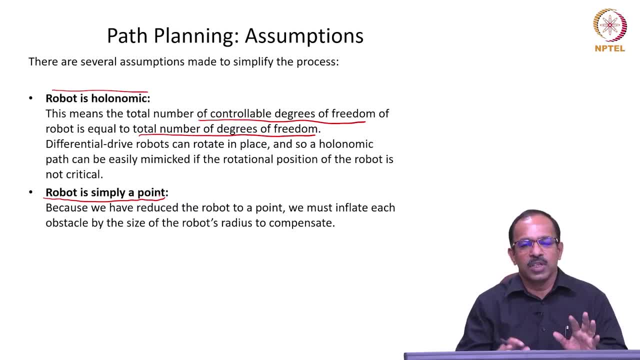 point, so that we can plan the path without worrying about the size of the robot. This, again, a simplification of the actual scenario. but we assume that the robot is a point and, in order to take care of that assumption, what we do is we will enlarge the size of the. 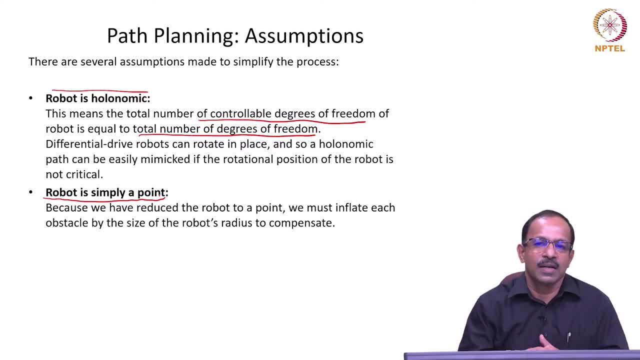 obstacles in its environment. with the size of the robot, That is, we inflate each obstacle, but the size of the obstacle will increase to a certain length- the size of the robot's radius- to compensate. So what does it mean? is that, if you have 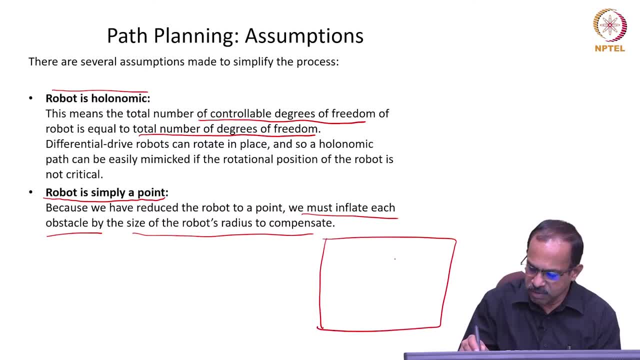 a scenario like this and suppose there is a an obstacle here and we have a robot of this diameter size, this is the robot, this is the robot and this is the obstacle. Now we assume that the robot size is 0,. I mean, there is no, it is a point, so there. 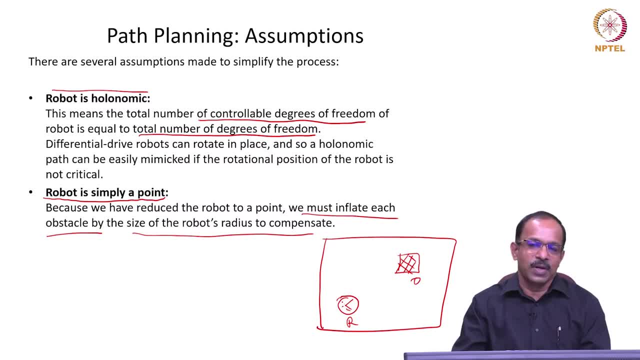 is no actual radius for the robot And to take care of that simplification, what we do is we will assume that the robot, this obstacle size, is bigger than the actual obstacle size, So we will actually add the radius of the robot to the size of the obstacle and 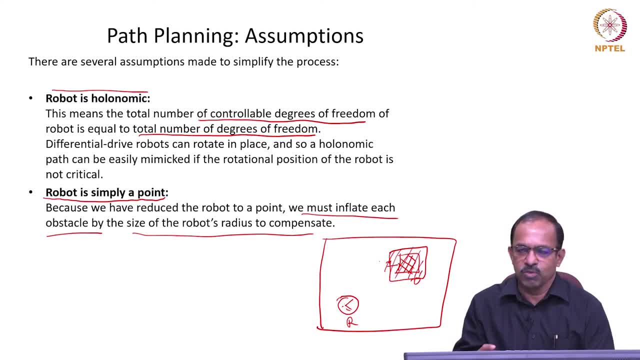 we will assume that size of the obstacle is this. So we will assume that the size of the obstacle is this. So we are actually inflating the size of the obstacle in order to take care of the size of the robot So effectively. though we are assuming it is a point, we ensure that 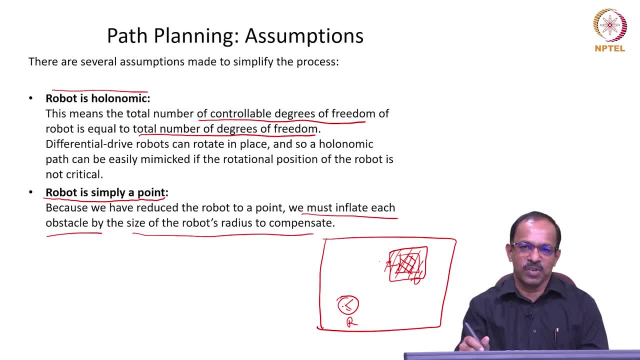 the robot will not really go and hit the obstacle because of its size, because the obstacle size itself is enlarged. So this one we call this as the configuration space, where we configure the obstacle with the size of the robot. So we call this the configuration. 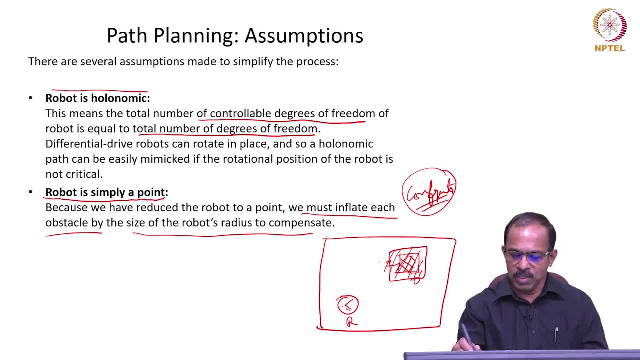 space of the robot. So the actual space will be will be having a smaller obstacle, but in the configuration space we assume that the obstacle sizes are enlarged in order to take care of the robot size. So that is basically the two assumptions that we make in planning for the. 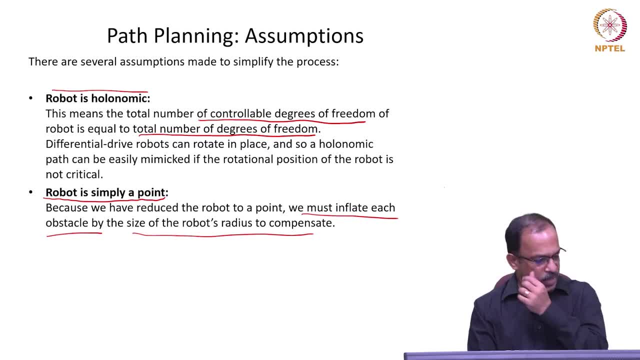 path in path planning of the robots. Now, as I mentioned, there are multiple methods for path planning And the path planning of the robot is basically the same as the path planning, The two most important one, basically the classical methods. There are many other. 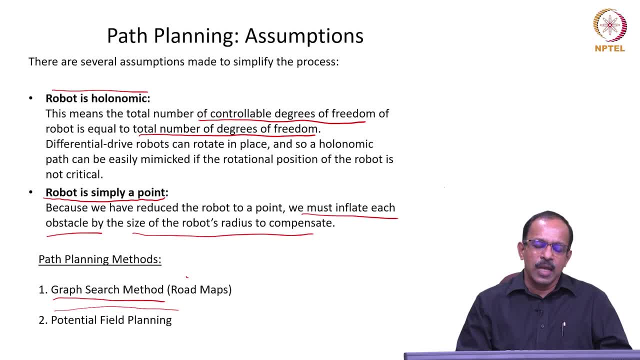 new methods are being proposed by researchers, but we will talk only about the classical methods. So the first one is known as the graph search methods. The second one is the potential field planning. So both are for path planning. In graph search methods, what? 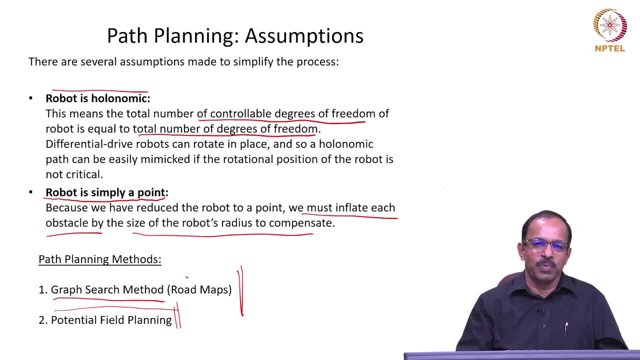 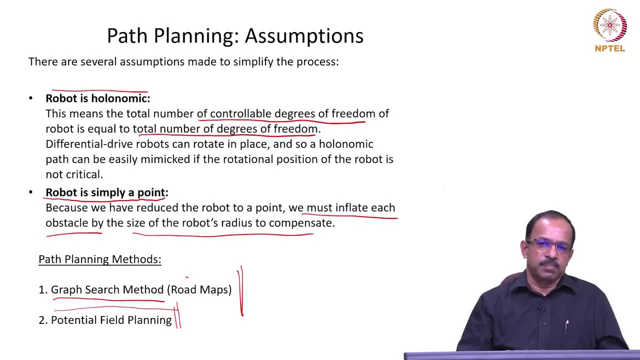 out which is the shortest path. In potential field path planning we do not go for a construction of a graph or anything. We assume that the obstacles and robot has got some properties and there is an attraction and repulsion and that actually represented using a potential field. and then we look at the this field and then decide which. 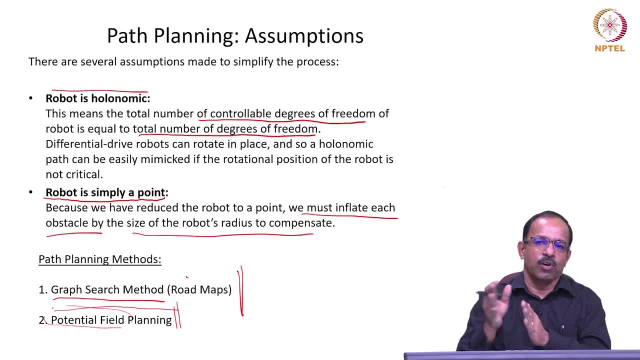 path will be having the lowest potential and then go along with that path. So that is basically the potential field method. We will look into these two in detail. So the first one is basically known as the graph search methods, or sometimes it is known as 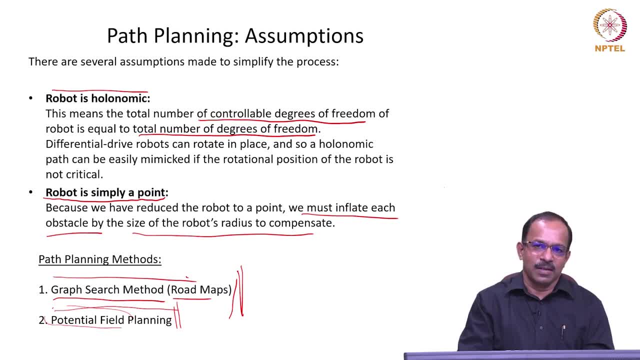 roadmaps also, Since, primarily, as you know now, if you use Google map or any other such algorithms, you can actually plan your route from one place to the other place in the map. So you can actually plan your route from one place to the other place in the map. So 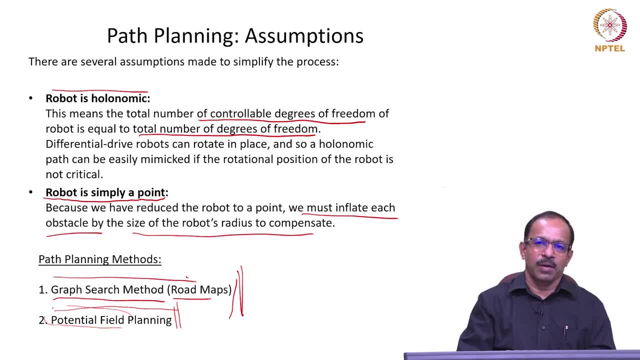 you can actually plan your route from one place to the other place in the map. So if you want to go from your institute to a market or some other unknown location, you can search in the Google map and then Google map will show you multiple paths. So 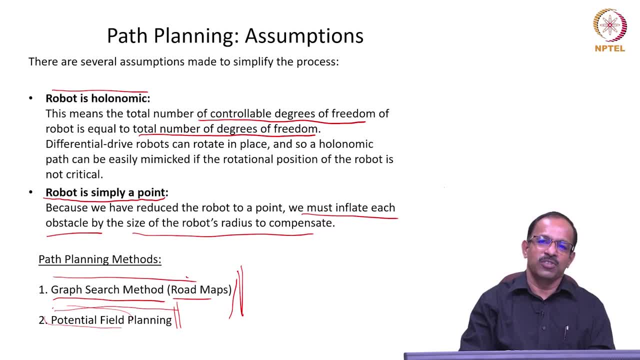 that is basically. it will show you all the possible ways in which you can reach. So that is basically. it will create a roadmap to reach the location. There will be multiple. you will see that it is not a single one. there may be multiple. 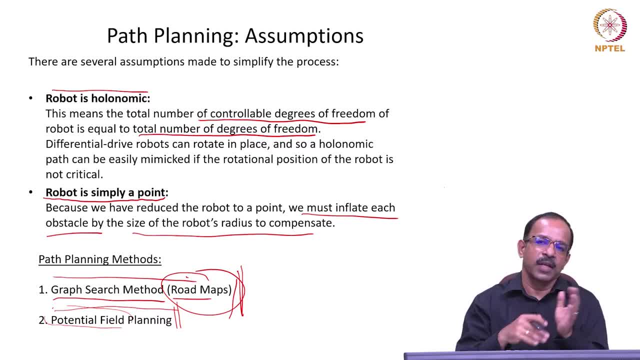 paths it will be giving you. So that is the graph and then, within the that multiple paths, you can search, or you can decide which one to take, based on the distance to be covered or the time to be taken, or the there is a, it is a highway or not, or there is a toll, or 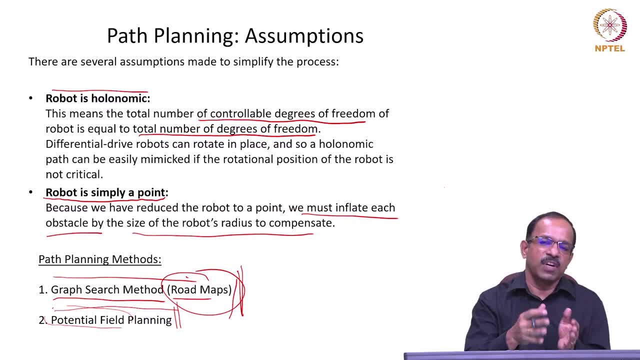 not, So there are different criteria you can use. This is same thing what we do here. also, we try to find out all the possible paths and then see which path is the best for your application. So there is there are two stage stages involved in in graph search method. So 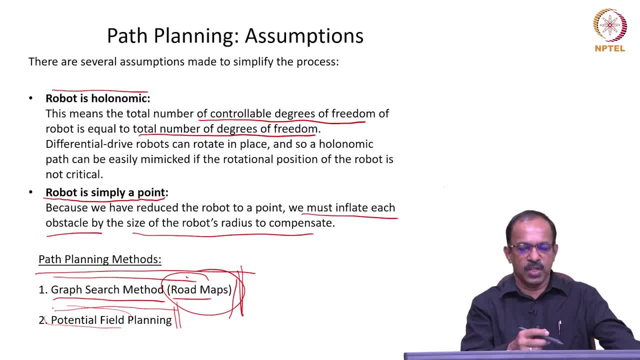 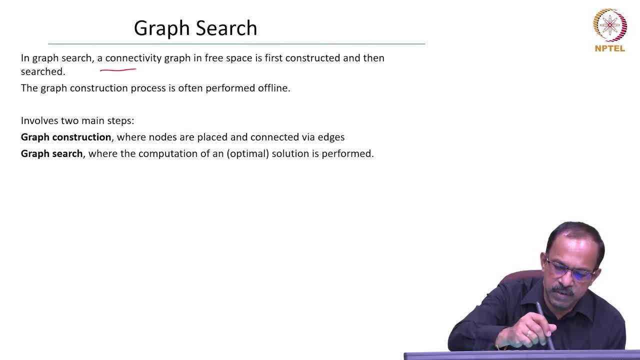 we will first look at the graph search method. So we will first look at the graph search method And then we will go to the potential field method. So what we do in graph search is a connectivity graph in free space is first constructed, So we will try to construct. 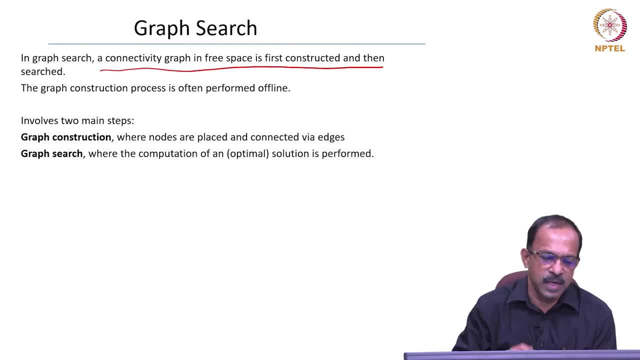 a connectivity graph in the free space and then we search in that graph the best path. So therefore it will be normally done offline. That means you have the all the information about the environment, the size of the obstacles and the location of the. 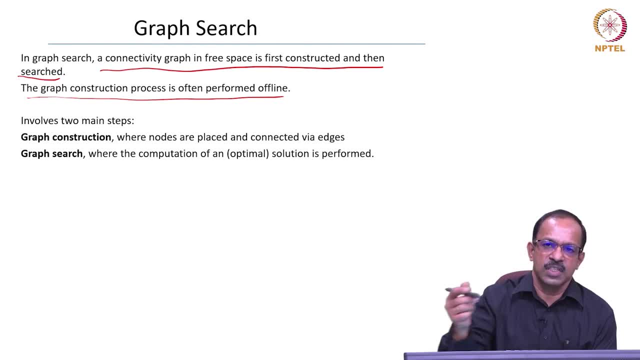 obstacles, all are given and you know the initial position and the target position. Then what we do, we will try to find out all the connectivity between the starting point and the goal point And then, once you have this connectivity graph, you search within the graph. So that is the procedure using: using graph search, That is. 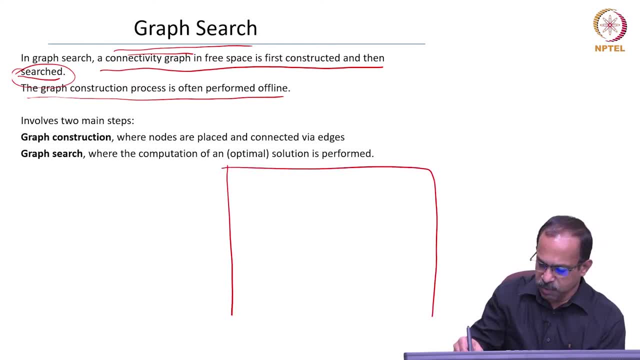 if you, you have a, a map already given, because it is an offline method, and then this is your start point and this may be your goal point, And you will see that there are obstacles on its paths. So assume that these are all the obstacles on the path. it is on the configuration space. So 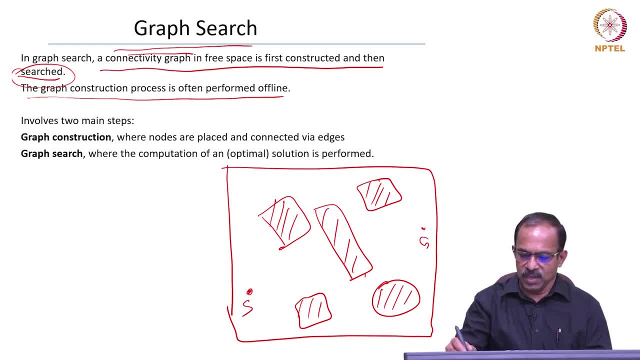 we assume that the robot is a point and it can actually move. Now what we need to know is what are the various paths existing between the start point and goal point So I can actually identify a path like this. I can go like this: 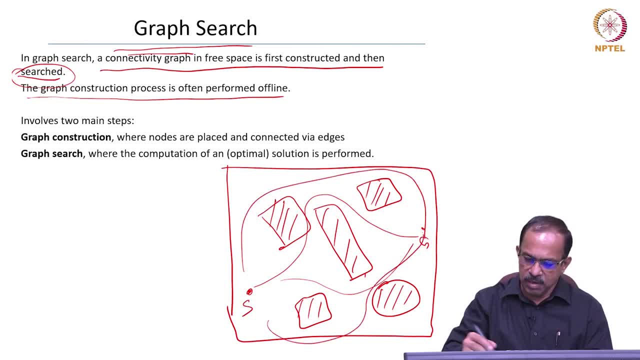 I can go like this. So there are multiple ways in which you can actually reach. So all the potential connections from start to goal will be the graph. So once you have all these, then we call this as the graph. So we call this as the graph. So we call this as the graph, So we 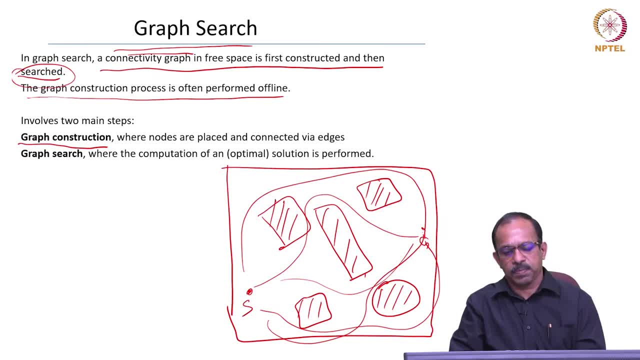 create a graph- we call this as graph construction- And then this graph. within this graph you do the search and then check which one is the shortest or the less time taken or less cost of travel. that is basically how you do it. So you create a graph first, So 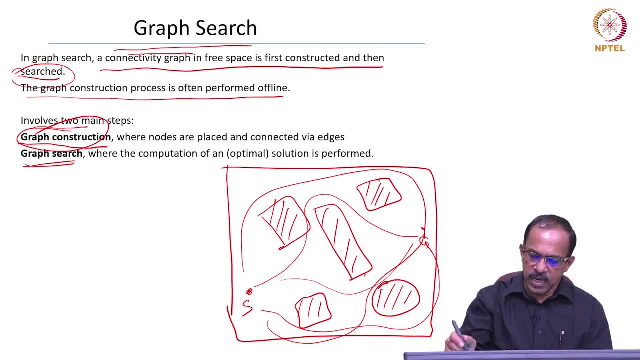 construct the graph first And then, within this graph, you search for the shortest path or the most feasible paths. that is the graph search methods And, as you can see here, we need to have some kind of a formal procedure to do this. 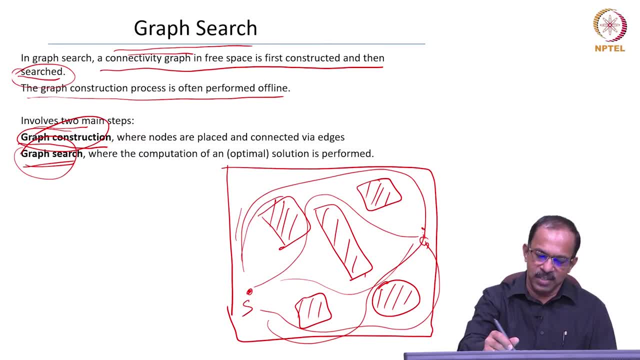 otherwise you do not know whether to go like this or like this, or what way we actually decide which path to be taken. So we create some kind of nodes and then adjust to connect the start to goal position. So that is the most basic way of doing it. we need to connect. 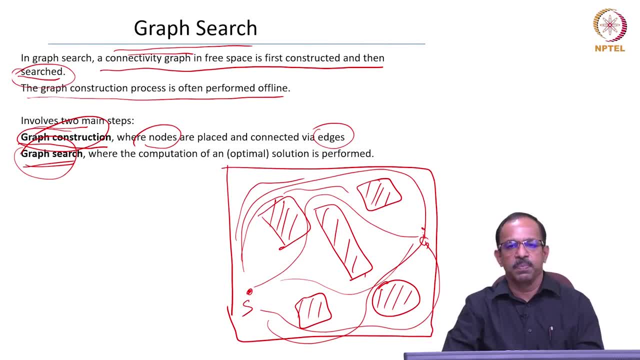 create some kind of nodes and edges so that it can actually pass through this edges to reach the goal point. So again there are different methods proposed in the literature to create the graph. So first we need to have the graph created and then do the search. So in the graph search method, 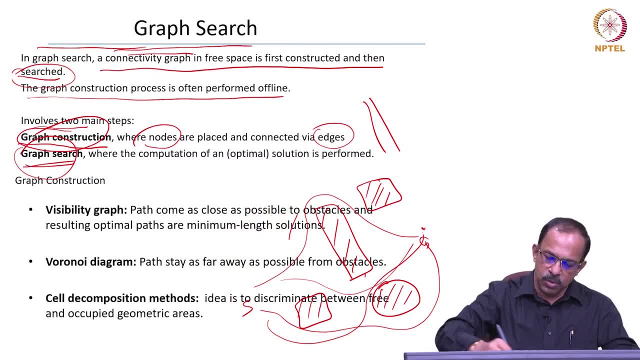 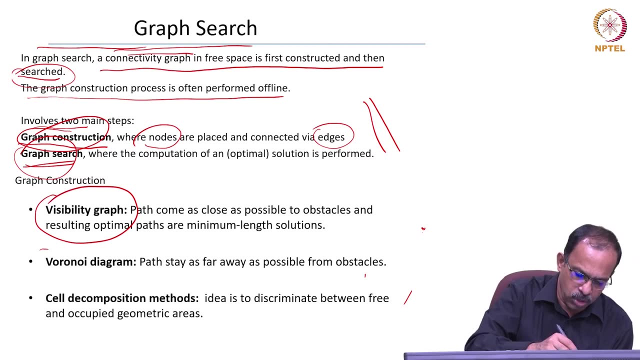 we will have multiple methods to create the graph and to identify all the potential paths existing. So some of the commonly used methods are known as visibility graph, Voronoi diagram and cell decomposition methods. As I mentioned, all these are offline methods. 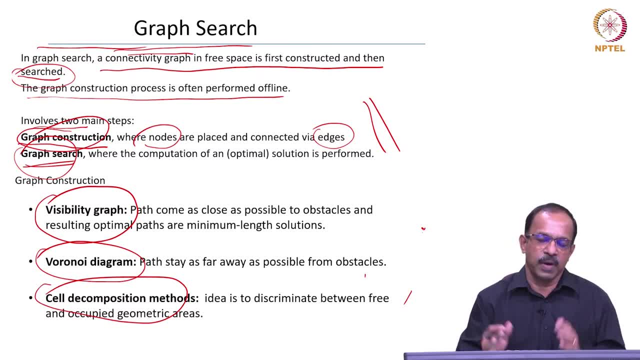 So we do not do it online, we do not do it as the robot moves. we will plan all everything offline And then we will use the path to the robots, And each one has got its own advantages and disadvantages. A visibility graph comes as close as possible to the obstacles and resulting 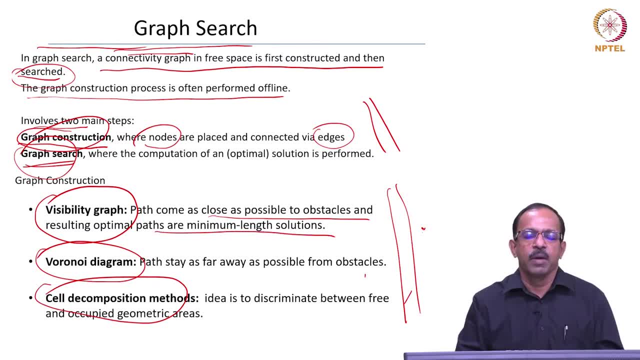 optimal paths are minimum length solutions. So we can actually get a minimum length solution as the robot will actually go very close to the obstacles and reach the target without hitting the obstacle, But in the other case- Voronoi diagram- it will try to keep as much as. 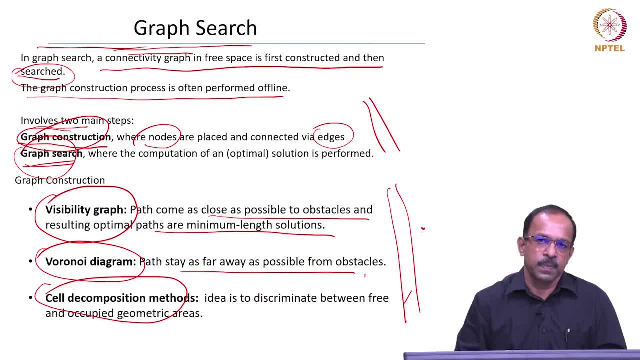 away as possible from the obstacle. So this path need not be the shortest path, but it can be a path where actually the safety will be much more conveyed to the visibility graph. And then there is another method, called cell decomposition, where actually it will try. 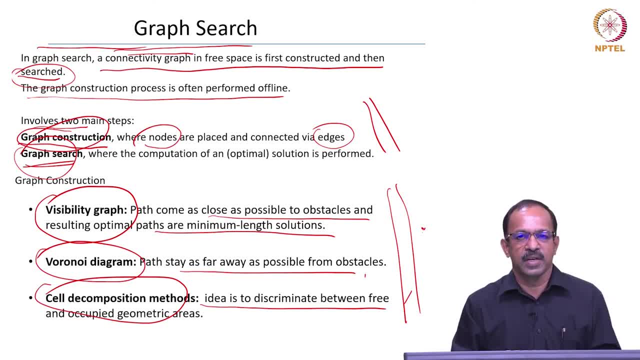 to distinguish between free and occupied cells and then try to identify all the free cells through which the robot can pass and then find a path, Then create a graph and then find out the best feasible path. So let us look at the visibility graph first, and then we go to the once you understand visibility graph then. 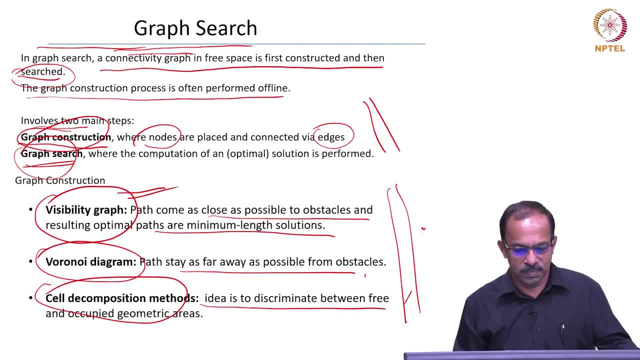 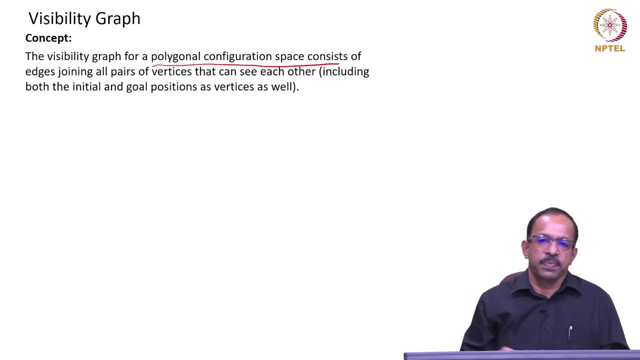 other methods will be much more easier to understand. So visibility graph for a polygonal configuration space. that means we assume that the configuration space has got all polygonal space. So what we will do is we are going to do a actions analysis with the RV случай model. 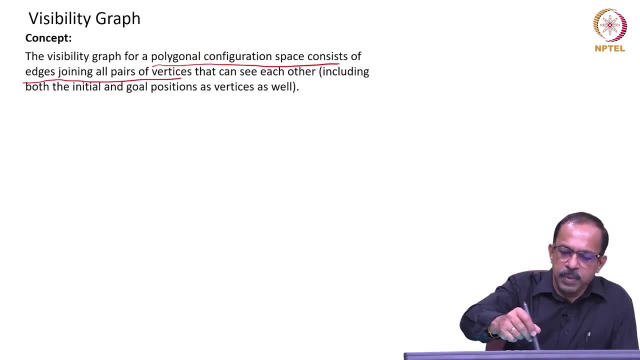 which is quite easy, and靠, and for us, we will model the we would imagine, looking at the delay, the goal point. So we consume this as a node or a, we consider this as a vertex, and then we know that there are obstacles, So we assume that these are all the obstacles there are. 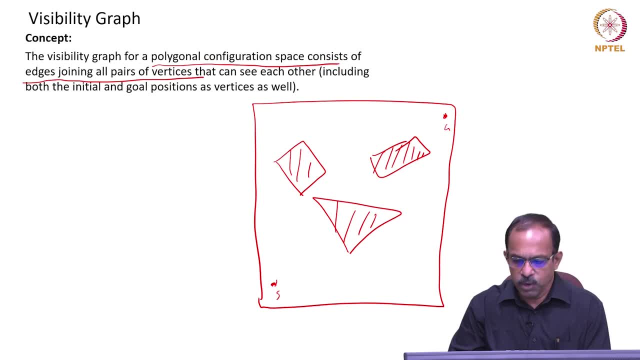 configuration space obstacles, so the size has been increased. Now what it will do? It will connect using edges all pairs of vertices that can see each other. So now this can actually see this vertex, So I connect using the edges. 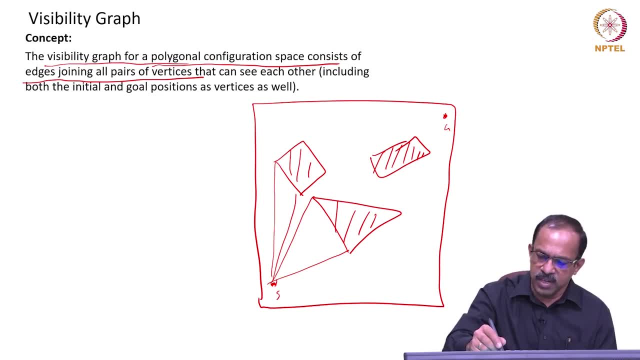 so I can see all these from here, So I will connect it then. this can see here. it can see here. it can see here. it can see this. Similarly, this can also see. this can also see here can see. this can see. there are always, there are multiple ways in which it will see. So 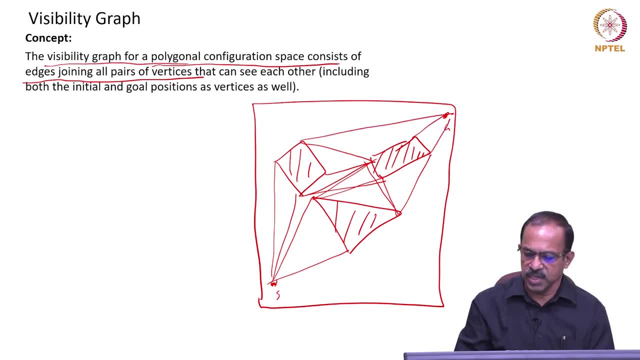 it can actually see this one. similarly, this also can see here. So now I will connect. these are all the edges. these are all the edges connecting the vertices, vertices which can each see each other. these are the vertices, So it cannot see. so these are all the edges that can connect. 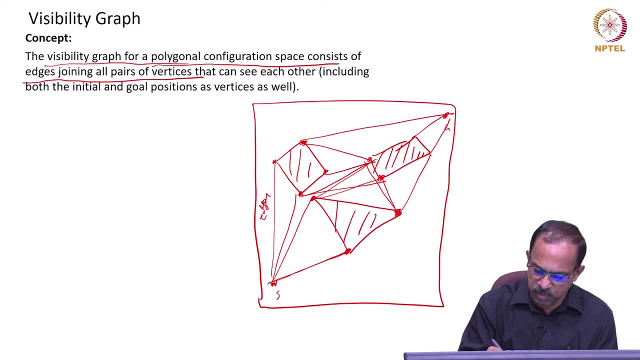 Now we can see that this robot can actually start from here, go up to here and then pass along this, and then go along this and then go from here to reach this point. So this may be a potential path, Since the actual obstacle is. 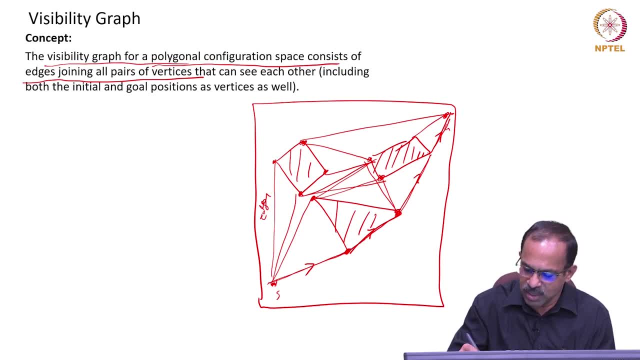 smaller than this. so even if the robot is moving along this edge, it will not hit the obstacle because there is already. the actual object or obstacle may be only this much size. So that is the assumption here and therefore the robot can actually take a path from here to here. 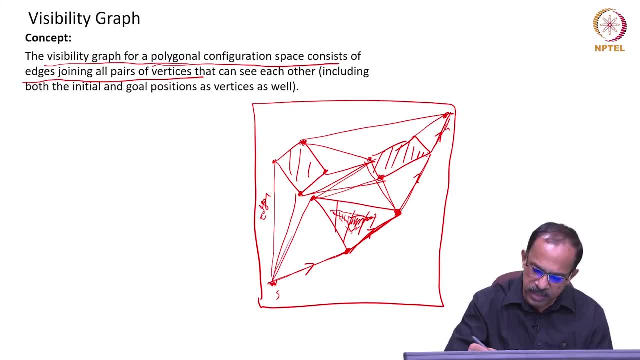 from here, then here and then reach here. Or it can go like this: then pass here and then going this and then reach here. So like this, there are multiple options for the robot to move. So these are all the potential option for the robot to move from: here and here or here. 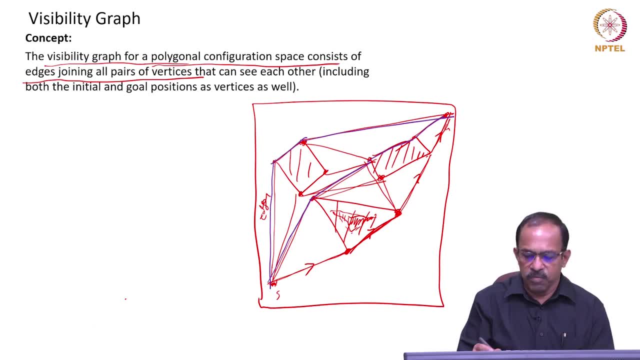 here. So this is basically known as the visibility graph. So all the visible edges, the vertex, are connected using edges and then we get a visibility graph. So we have multiple paths possible. So that is the first stage of graph construction. So 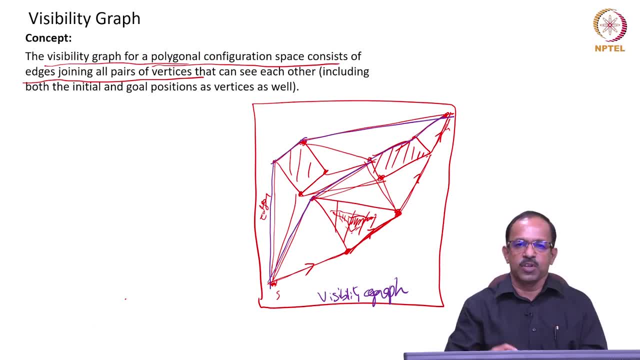 we have constructed a graph which shows multiple paths for the robot to go without hitting the obstacle and reaching the target. So that is the first stage in visibility graph. It is a polygonal configuration space consisting of edges joining all pairs of vertices. 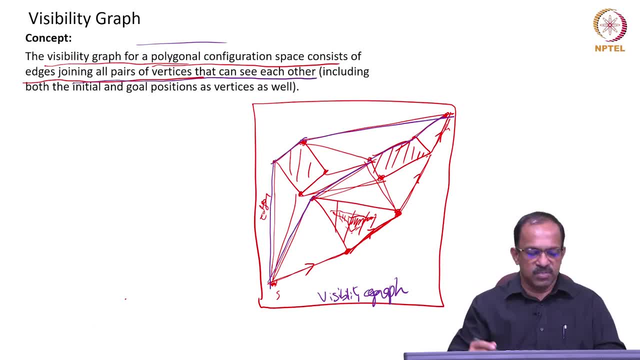 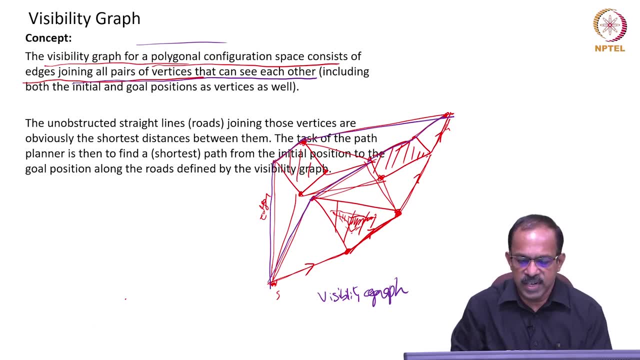 that can see each other, including the starting and goal points. So that is the thing. Now. the unobstructed straight lines joining those vertices are obviously the shortest distance between them. The task of the path planning planner is then to find out the shortest paths. 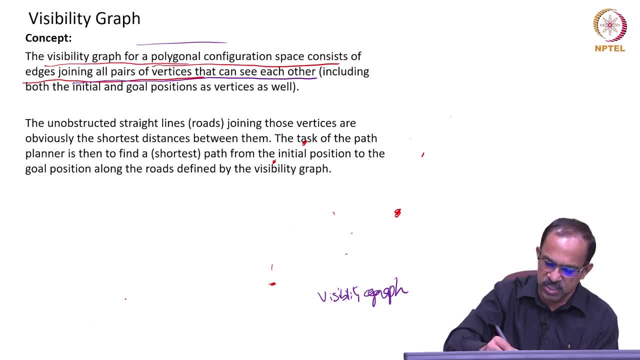 from the initial position to the goal position. So that is the second stage. First stage is to construct the visibility graph. So once a graph is constructed, then you can search within that graph to find out the shortest path, or whatever the criteria you set, you will be able to. 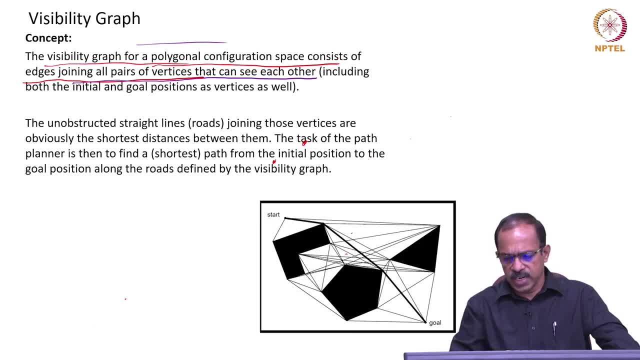 find out the paths. This is the one which I already explained, So you can see there are multiple paths possible like this, like this. So one of these may be the shortest, but we need to find out which one is the shortest and then that it can be done using a. 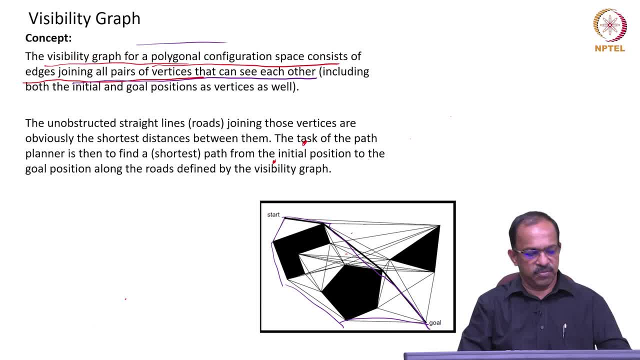 again a search algorithm. So first one is creation of the graph, And it is a simple process and which can be done offline, and then, once you get the offline data, you can actually feed that coordinate points to the robot and the robot will be able to. 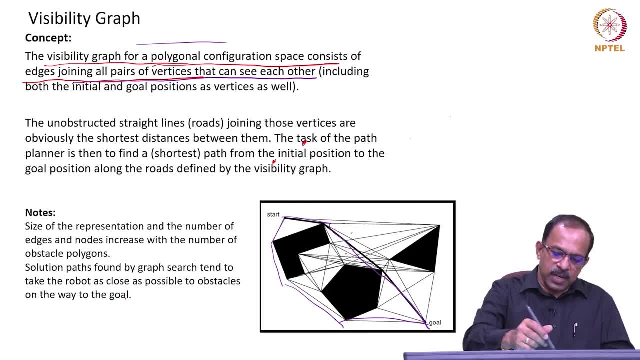 go along that path. But the difficulty is that with the number of obstacles- as the number of obstacles increases- you will be having a much more complex graph. It may find it difficult to handle it. Solution paths found by the graph search tend to take the robot as close. 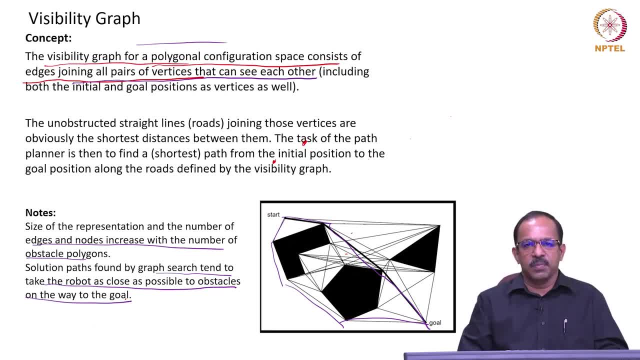 as possible to obstacles on the way to the goal. So that is another disadvantage here, because, as you can see here, the robot may be going very close to the, for example, in this path, you can see, it is actually very close to the obstacle. Though it is, the size is enlarged, it maybe still. 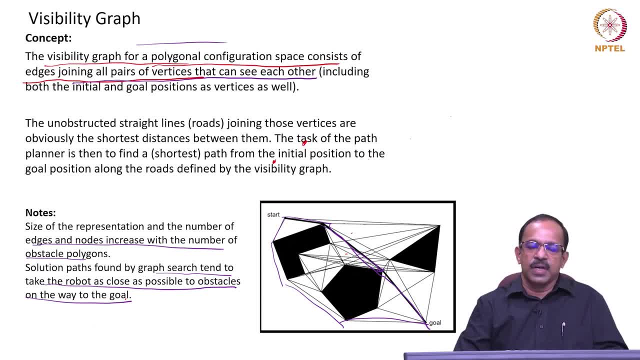 close. if there is a small error in the robot's position, there is a high possibility that the robot may hit the obstacle. So we need to take enough precautions to avoid that situation: Either increase the obstacle size more than the size of the robot or give some clearance in all the paths. 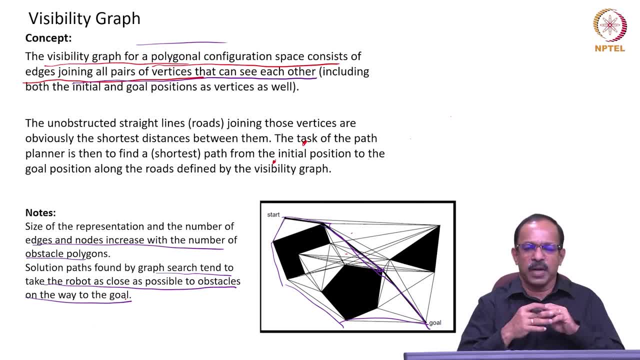 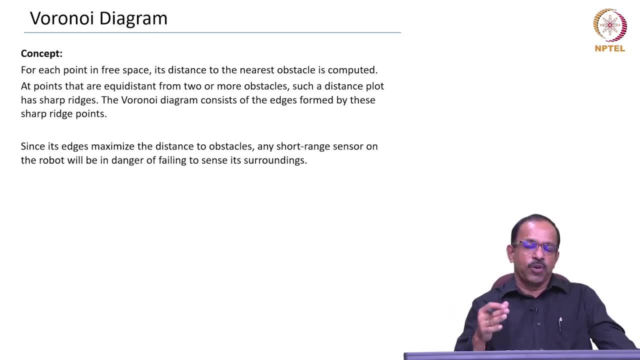 to be away from the obstacle. So these are the practical issues we need to understand when we do the visibility graph method of path plan. So to avoid this problem of the robot going so close to the obstacle, there is another method called Voronoi diagram methods. So in the Voronoi diagram the robot will be 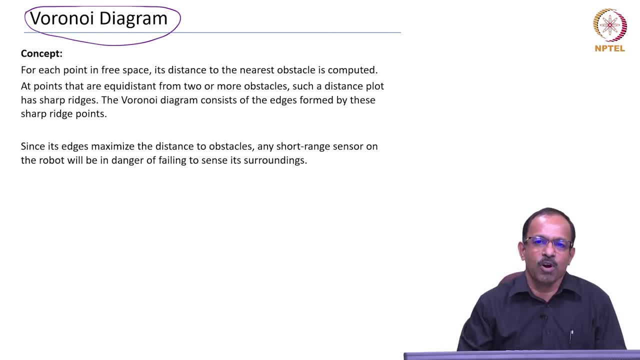 moving as much away as possible from the obstacle. So that is basically the method of Voronoi diagram. So what it will do it for each point in free space- is distance to the nearest obstacle is computed and that points that are equidistant from two or more obstacles. 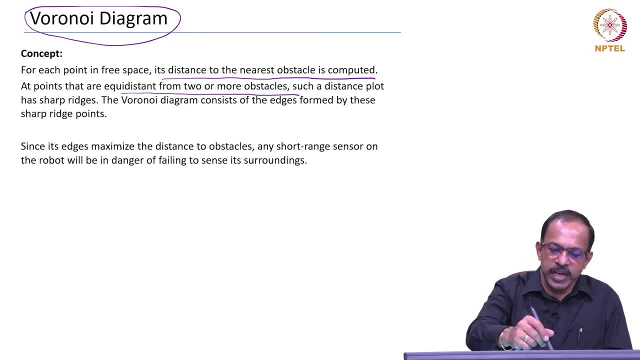 that such a distance plot has sharp ridges. Voronoi diagram consists of the edges formed by these sharp ridge points. For example, suppose this is the area and the robot is initially here and there is an obstacle like this. So what it will do is it will try to find out what is the space in this point. the point. 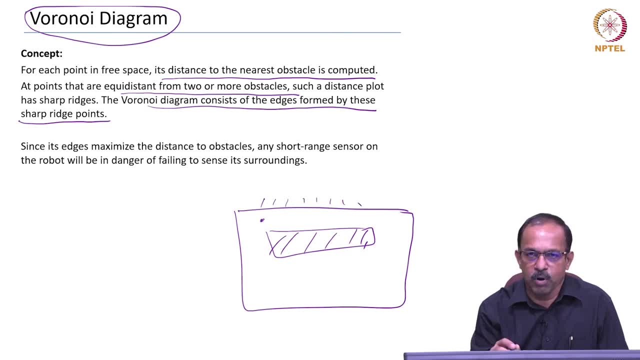 which is equidistant from this one. this is again a boundary, So there is a kind of an obstacle and between these two. So it will try to find out a path which is equidistant from these two, So it will try to find the points which are equidistant from these two. 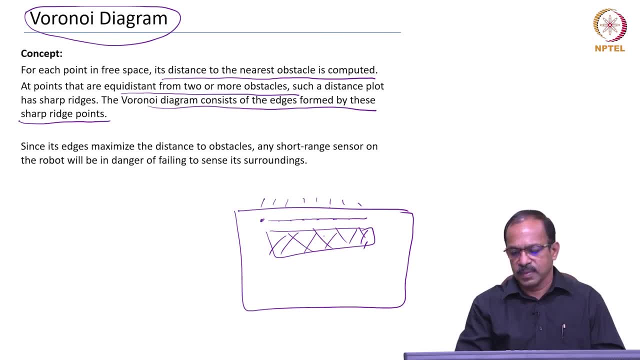 and take that as the possible path from here to here. And that is basically the Voronoi diagram methods. So once you can identify all those, depending on the obstacle and the boundaries, you will be able to get all the path which are equidistant from the obstacle. So in this case it will be: 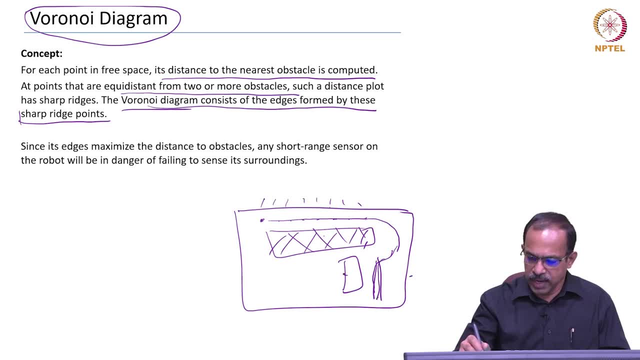 like this, equidistant from this one and this one, and then it may reach here the target. So these are the possible ways in which you can think, or the possible paths which are equidistant from obstacles is basically the Voronoi diagram. So this is the Voronoi diagram. So 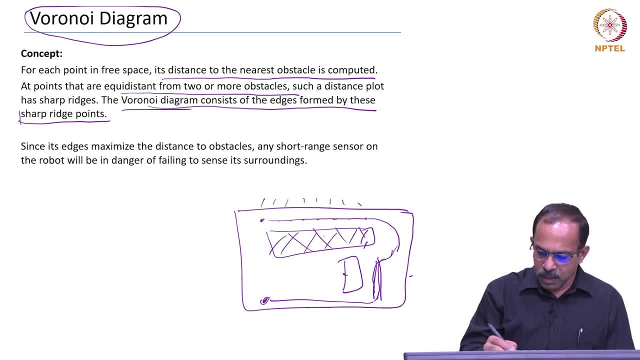 it is basically the Voronoi diagram. Of course, it has got its own limitation, because the sensors are when you use the sensors to identify the obstacles, So the, sometimes it may be, may not be able to identify the obstacle far away, It may not be knowing that there is an. 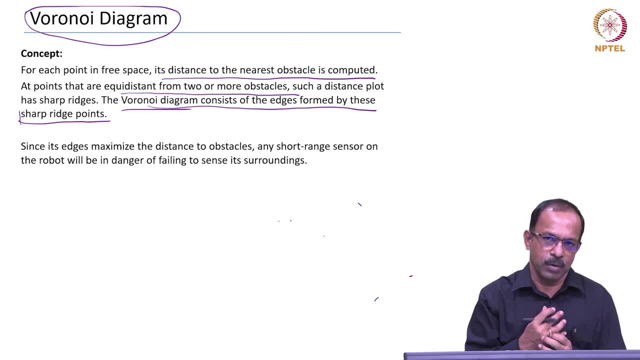 obstacle at the right location, that is, more in the online method, but offline method, since everything is known, you will be able to create a good Voronoi diagram and then use it for a plan. Ok, Thank you. Thank you very much. 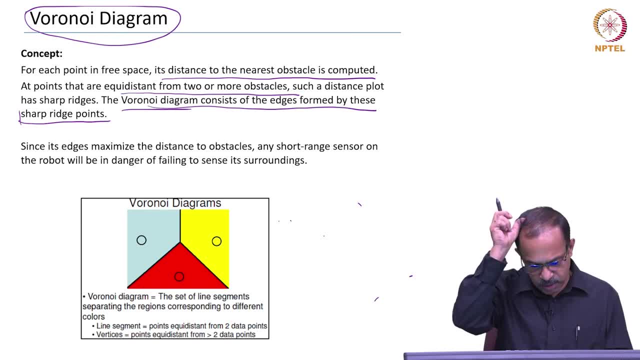 Thank you, Thank you very much, Thank you very much, Thank you, Thank you, Thank you. So this is again example of this fortnight method. So you can see that these there are. there is an obstacle here and there is an obstacle here. it will identify this as the shortest path. 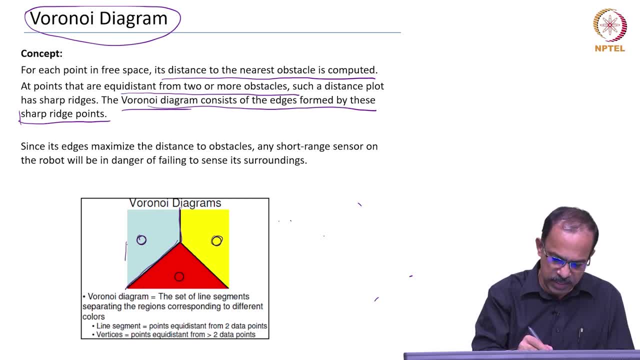 And similarly, this can actually be because now there is an obstacle here. sorry, there is a boundary here and here, so it will identify this as the path. So this way, you will be able to identify the paths, The set of line segments separating the regions. 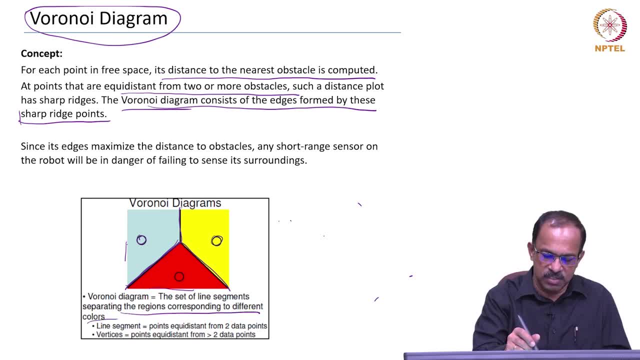 corresponding to different colors, So lines- this is in this case. it is different colors, So each color will be separate, So you will be able to get this as the possible path for the robot equidistant from all the place. 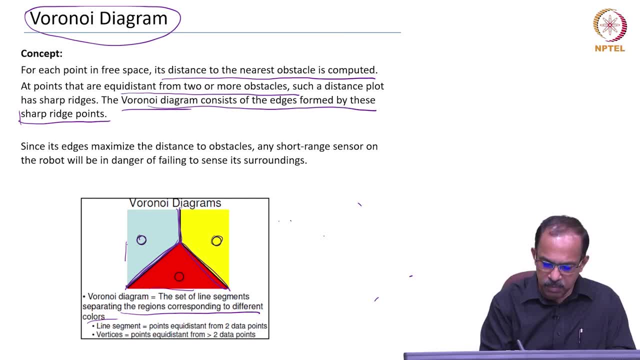 So you will be getting a line segment when you have from two data points. So if you want to take it from this one and this one, then it will be a straight line. But you have three conditions. So now this one, this one and this one. then this becomes a vertex as the. 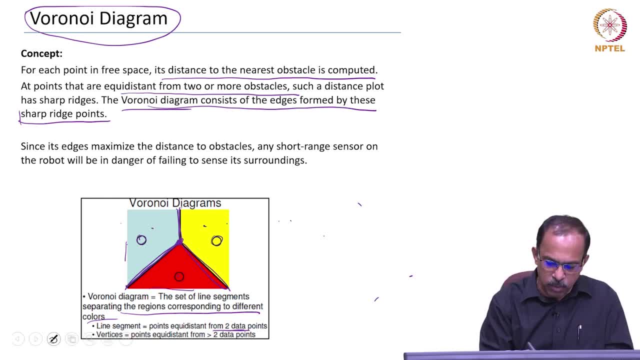 point which is equidistant from all the three, So vertices points equidistant from more than two data points, and only two data points. you will get a line segment, So this principle can be used in the construction of Voronoi diagram, and then you will be able to find out all the 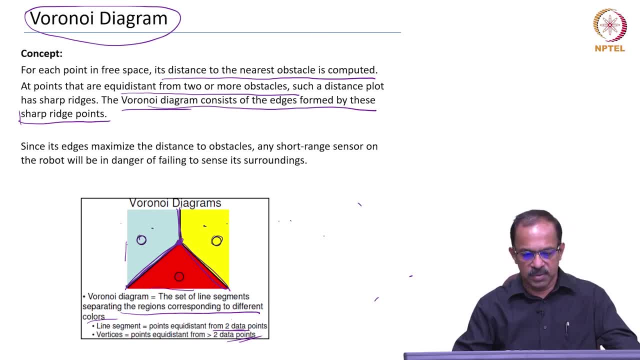 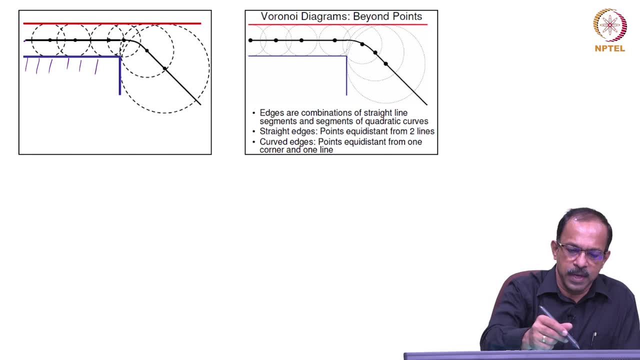 possible paths. We will take an example and then show you how this is done. So, for example, now if the robot is starting from here and you will see that there is an obstacle here and there is an obstacle here. So between these two data points you will be having a 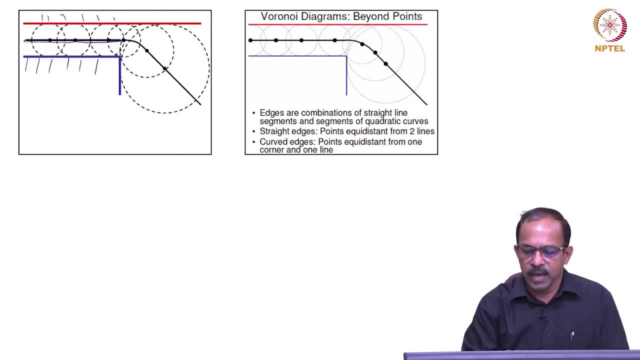 straight line And then you will be having from this edge and then this one, so that will be a curve. Then again, between this one and this one, you will be having a straight line. So this is the way how you can actually create. edges are combination of straight line segments and segments. 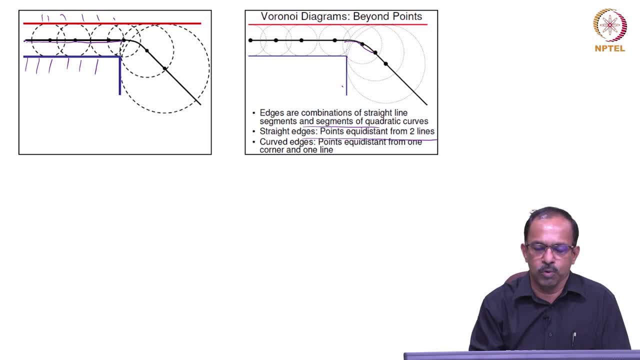 of quadratic curves And straight edges points equidistant from two lines and curve edges points equidistant from one corner and one line. So one corner and one line will be a curve, two data sets will be a straight edge And then this edges will be a combination of the like straight line and the 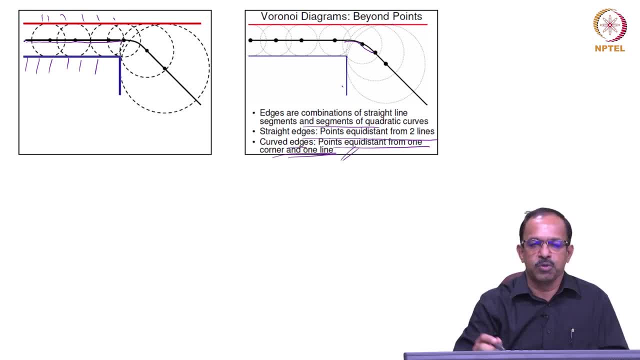 curves, curved edges, because you may be having situations where it is equidistant from one corner and one line, So in that situation you will be getting a curve also. So primarily you will be having this: edges as a combination of straight lines and curve edges, curves. So now look at this: 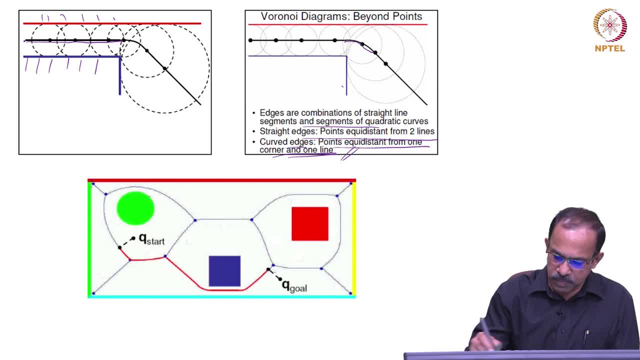 situation. So you have a area- I mean a space, configuration, space- with these are all the obstacles And of course, it will consider these boundaries also as obstacles. Now it will try to find out the all the possible paths And if it is, this is a Q.